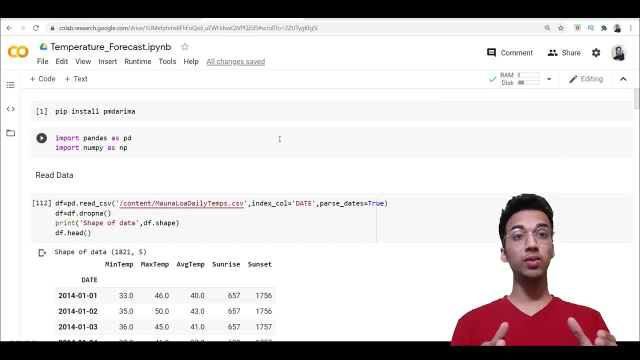 So hi guys, my name is Nachiketa and welcome back to my channel. In this video, I'm going to show you how to implement an ARIMA model in Python. In the last video, I covered auto regression, and I've already explained the theoretical concepts behind it, So make sure that you've seen those videos. I'm still going to give you a gist of it as we move along the code, So let's straight away get started. First step is to install a package called PMD ARIMA. I'm going to tell you why we're exactly using this- one of the most handy tools you can have for an ARIMA model- And after that we import. 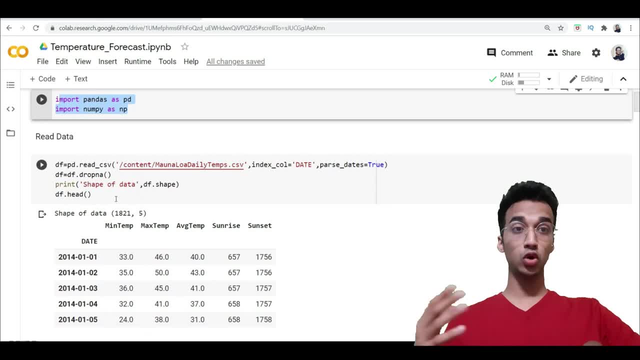 pandas as pd and ump as np, And first step is, of course, to read the data. So I'm going to read a data set which I've already imported onto my workspace. I'm going to leave a link for that in the description as well, And basically few parameters over here. index column is equal to: 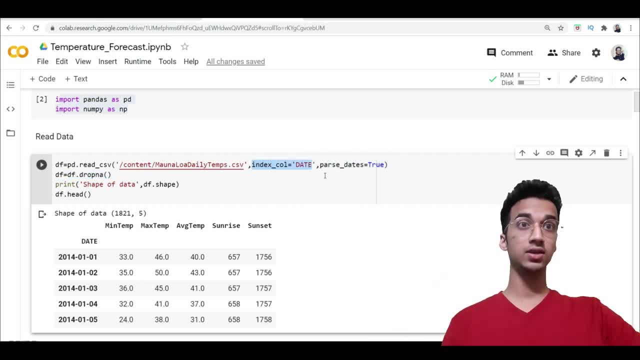 date, which basically sets the date column as its index right, and you have to write parse dates equal to true. This makes sure that pandas understand that it's dealing with date value, Otherwise it will treat it as normal strings. All right, After that. 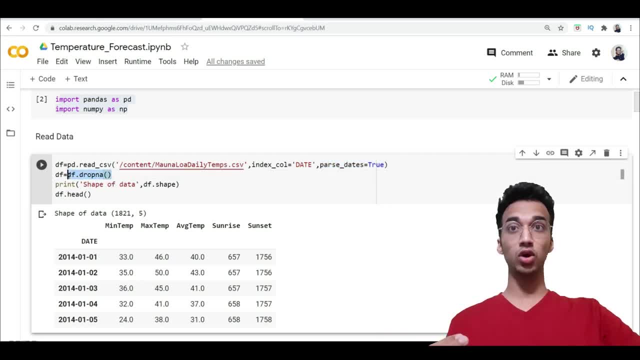 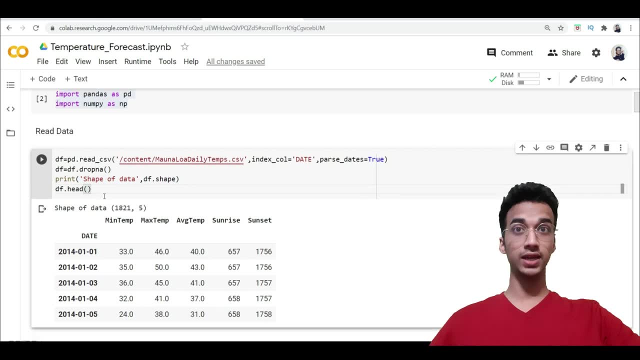 there are some missing values in the data set which we drop using df dot. drop any. After that you calculate the shape of the data set and print the first five rows just to see how your data set looks like, Right? So data set has 1821 rows and five columns, which 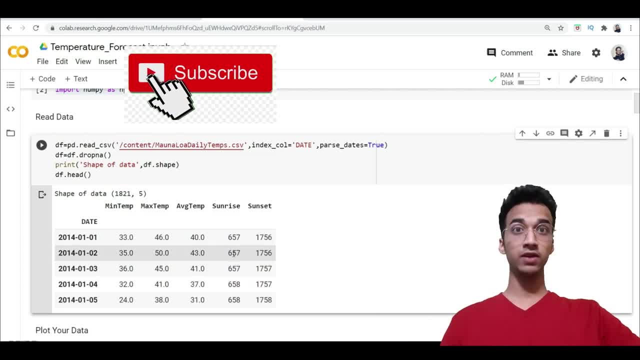 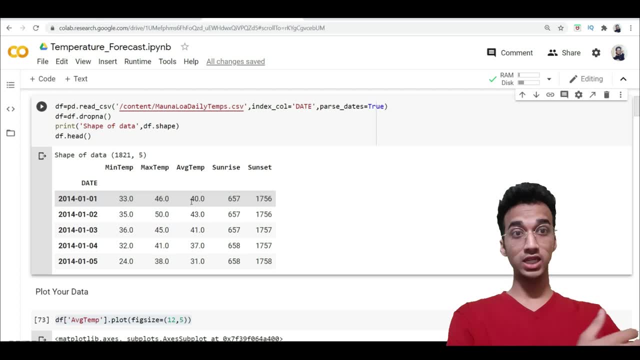 you can see over here, it has lots of values about a particular city. We're only interested in average temperature in this case. right, we're going to create a model to predict how the average temperature is going to change with respect to time. So first step is to 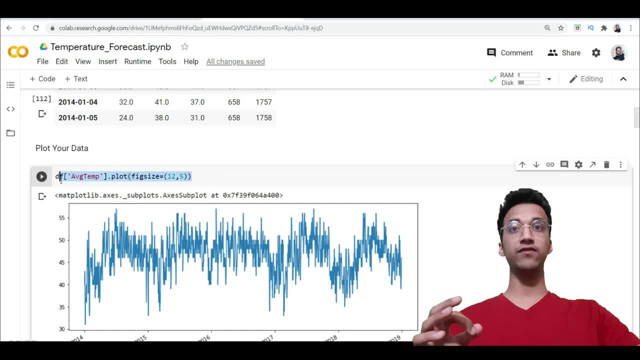 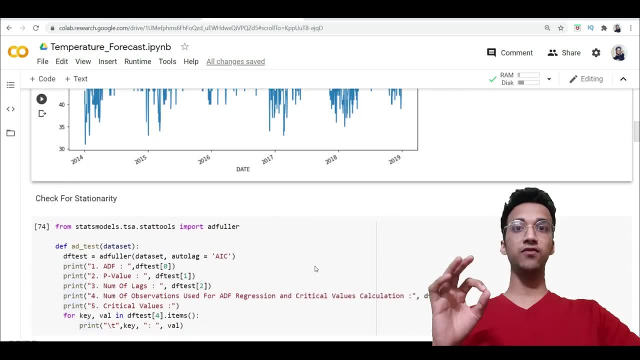 plot your data To get a feel of how it looks like. we do that using df, dot, plot, right, And this data set looks pretty much stationary, right, And you don't have to worry about that. we're going to run a fixed statistical test, like I shown in the previous video, which is called the. 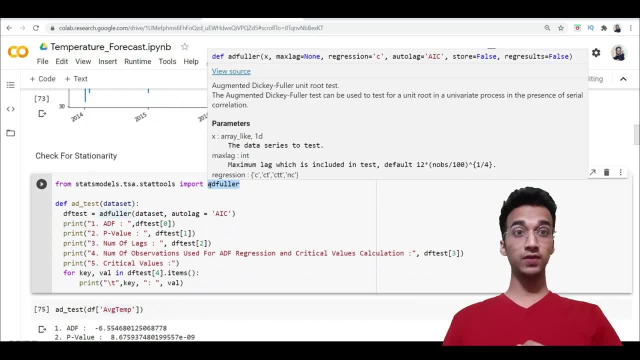 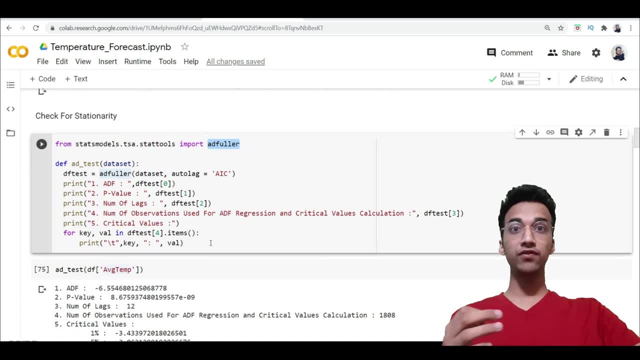 augmented Dickey field test. This is basically a test which returns certain statistical parameters which you can use to judge if a data set is stationary or not. So I've created a function over here And, as I said, this test is going to return an array of values, So we are capturing. 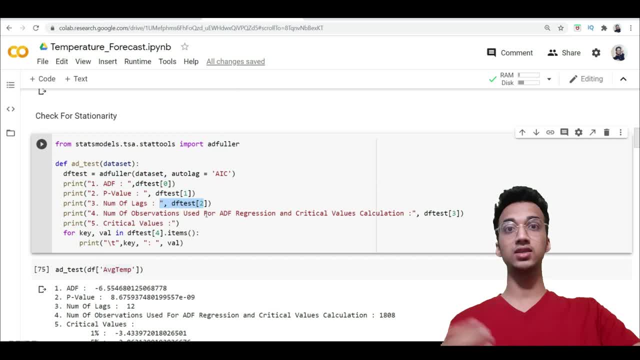 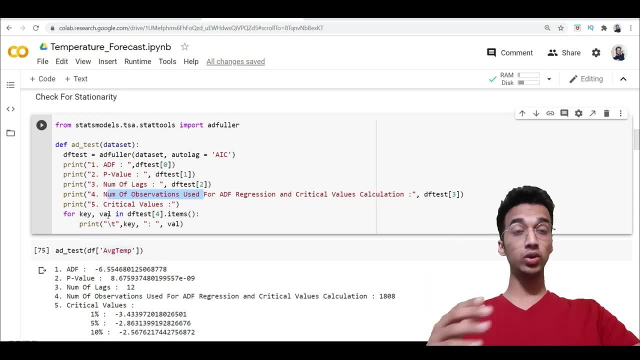 different values like the ADF, the p value, the number of lags, number of observation- right, But don't worry about this. we're not going to go in depth about what this test is. just you should know how to interpret the test right. So when I'm calling the test, 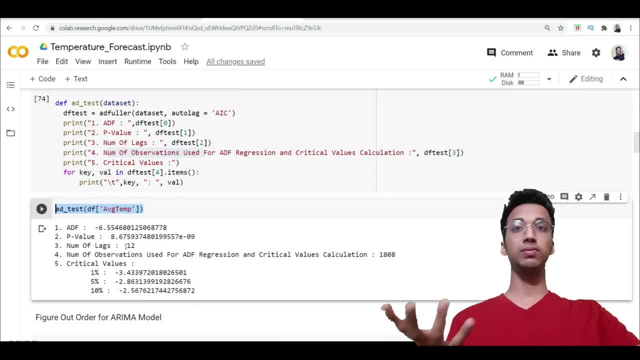 it returns a bunch of values, right? The only value that you need to be bothered about is the p value, Right? So, basically, if the p value is basically the probability, and it should be as small as possible If it is a higher value- say 0.8, 0.6,, 0.8,, 0.8, 0.8,. 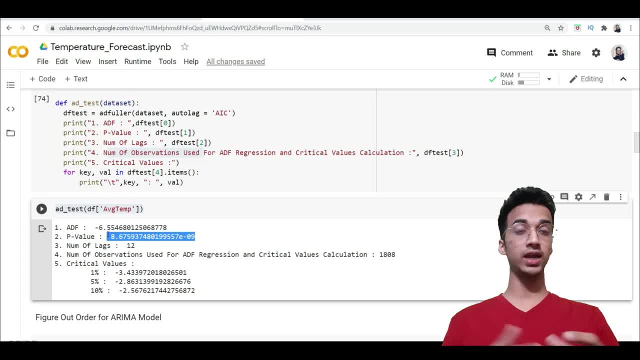 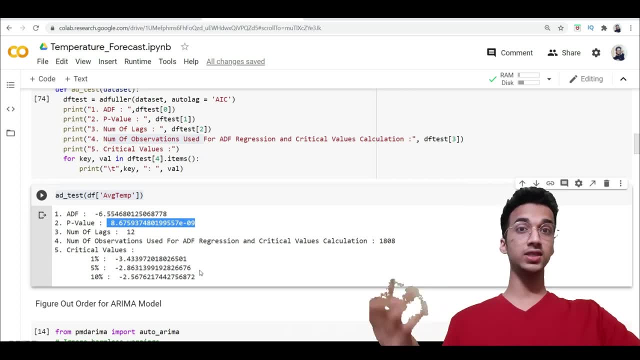 if it is a higher value, say 0.8,, 0.6,, 0.9,, that means your data set is not stationary, right? So ideally it should be less than 0.05, right? The smaller it is, the better. 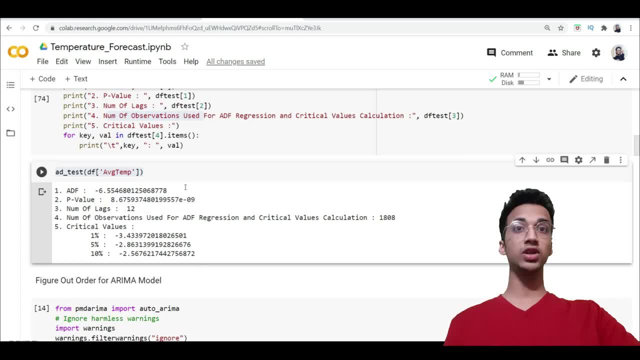 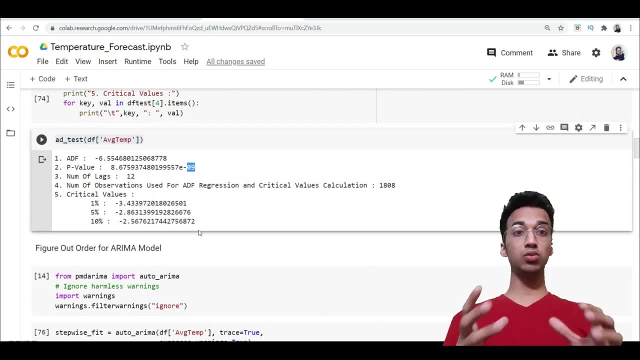 So this is a pretty small value, right, You can see. it is exponential raised to the power minus nine, right? So it's a pretty small value, which means the data set is stationary. we can proceed After that. the most important step in the ARIMA model is the figuring out. 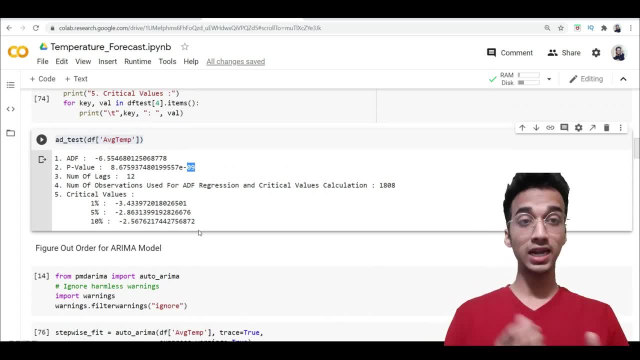 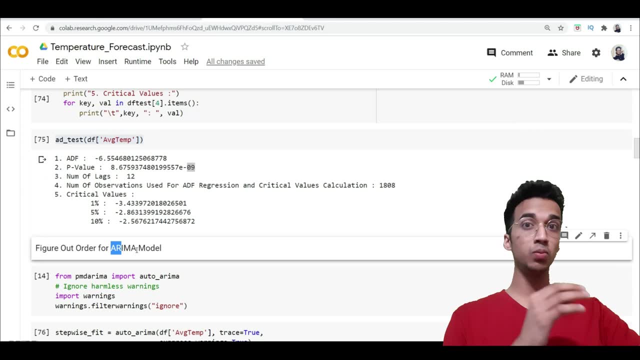 the order. Now I recommend you watch my previous videos on ARIMA. But let me give you a gist of that. The ARIMA model basically is divided into three parts. right, It has the AR part, which is auto regression, moving average and integrated. Auto regression basically uses the previous. 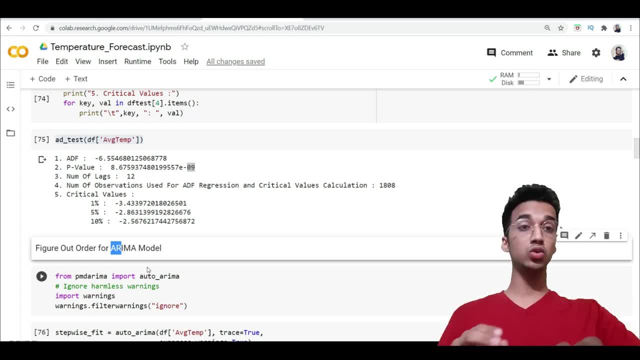 values to make a future prediction. Moving average is going to use the past errors to make a future prediction, And integrated basically means differencing right. So if your data is not stationary, right meaning if it has an increasing trend or it has a decreasing. 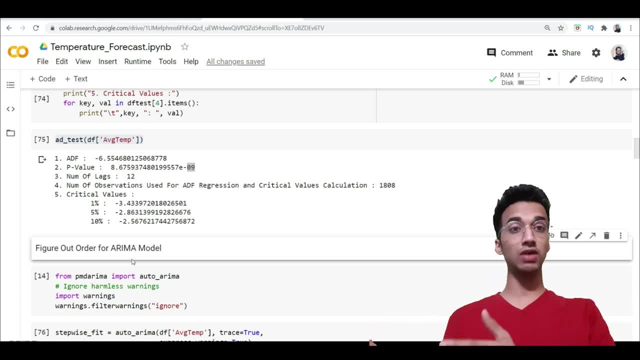 trend. you basically difference it right. you differentiate with the previous values to eliminate that trend. So for auto regression, if it has the second order, it basically means you're using the past two values to make a prediction. Similarly, for moving average, if the order is n right. 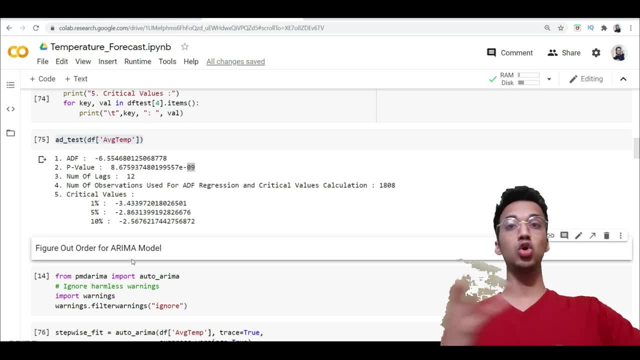 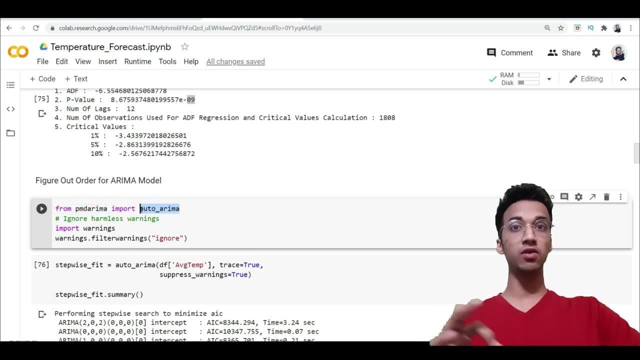 so it will use the past n errors to make a future prediction. So it goes on like this And we don't have to worry about any of that. The PMD ARIMA model takes care of everything. we simply import the auto ARIMA function right Over here. we're simply importing. 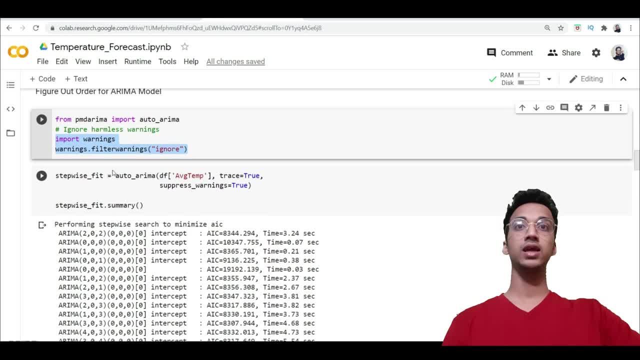 a library called warnings. to ignore any warnings that come up right- And here is where we call the function Auto ARIMA- we have to provide the data set over here. trace is equal to true. Basically, what it does is it will print out as it's iterating to every step right. So auto ARIMA. 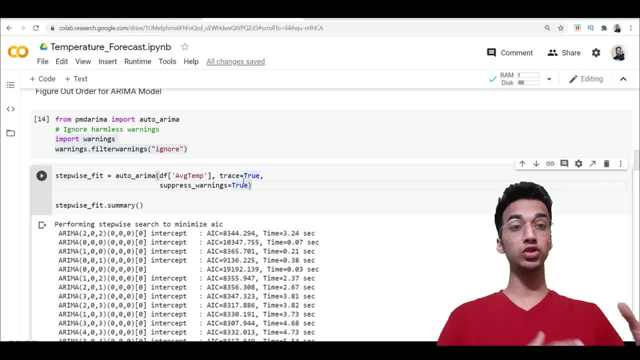 is basically going to try different combinations of orders- right 100,, 010, 012.. And for every model, every order, it's going to assign a score which is called as the AIC, And the goal is to minimize the AIC. So that's how it operates And it has a lot of parameters. 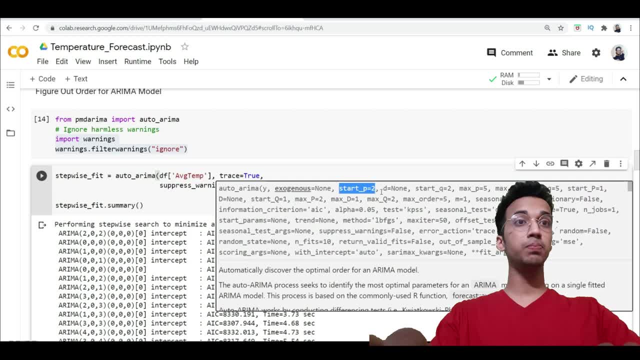 that you can check out, Like you can mention the parameters. you can check out the parameters. So that's how it operates And it has a lot of parameters that you can check out, Like you can mention the starting p value, right? So ARIMA order is basically named as pdq. 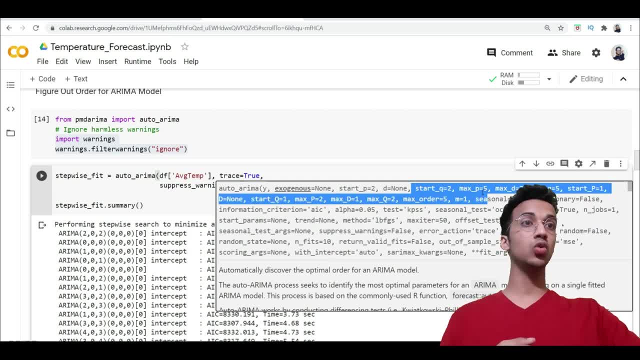 So you can mention the starting p value, starting q value, max p and max t value as well, And you can do this. if it's taking too long to converge, you can specify the starting and the ending points. So over here we run the auto ARIMA function and print out the summary. 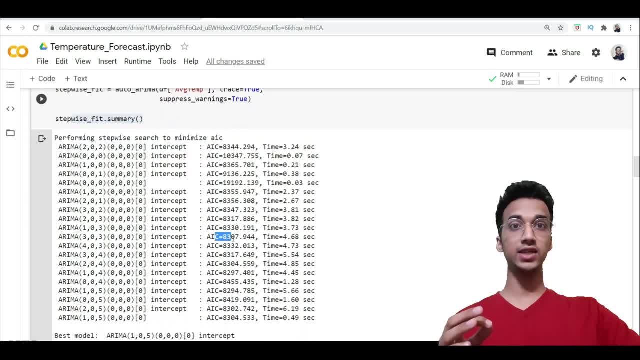 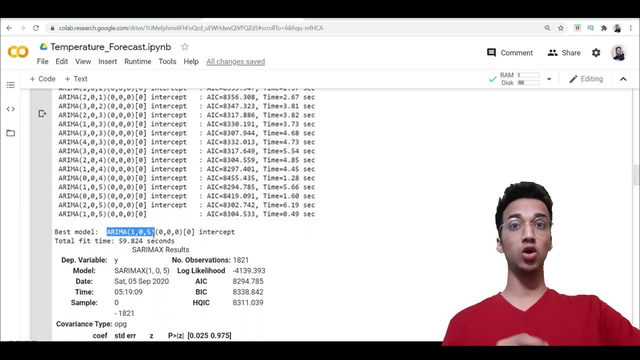 And it gives you different combinations of model with their respective AIC score. So basically, it's looking for the minimum AIC score, right, So it runs. it'll give you the right, so it is given over here, as the best model was of one comma zero comma five order. 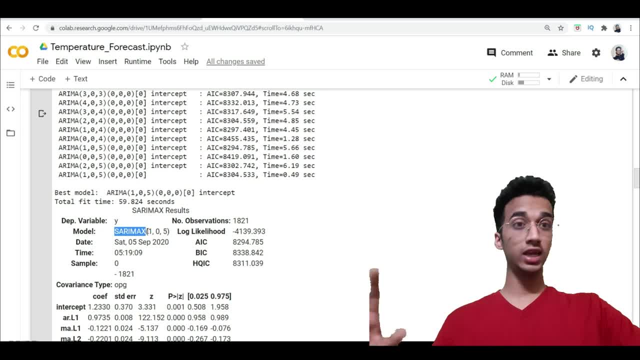 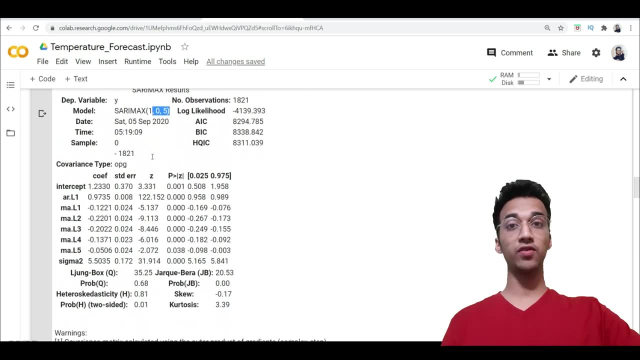 right, and i know over here it says sarima, but you can ignore that, right? so sarima is basically an arima model with seasonality right, and since there's no seasonality in our data set right, this is simply an arima model. so this is basically an arima model of order. one comma zero, comma five. 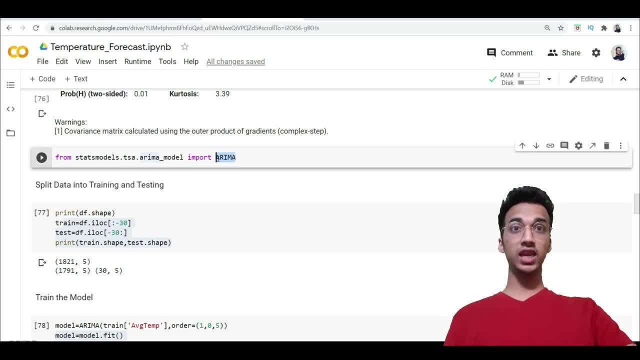 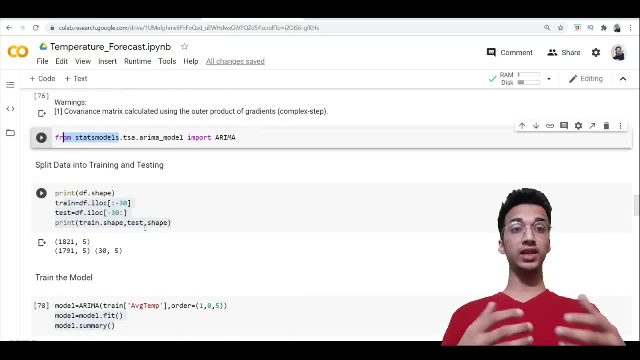 so now we begin with actually fitting the model right. we call the arima function from stats models all right. and the next step is to split the data set into training and testing. you'll train the model on the training section and just check if it's good or not on the testing set. 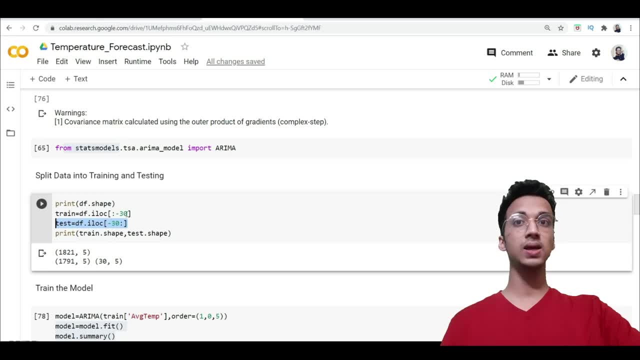 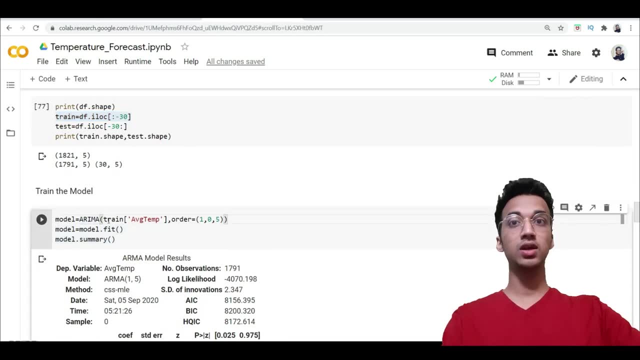 right, so we reserve the last 30 values as a testing section and rest of the data as a training section. all right, and to fit the models, you simply call the arima function and you give it the data set, which is the training section. you specify the order that you want. 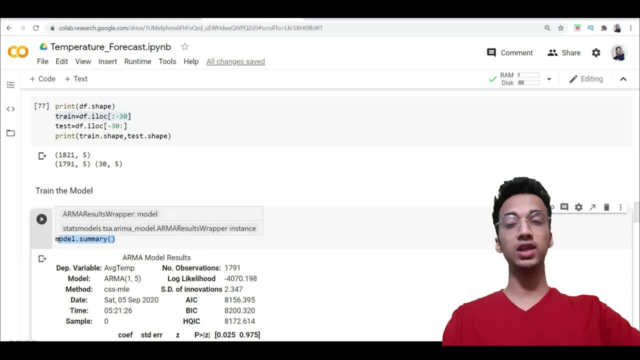 and you fit that using modelfit, and you can see the summary as well. if you want to see the summary as well, you can see the summary as well. if you want to see the summary as well, you can see the summary as well. you can see the summary as well. you can see the. 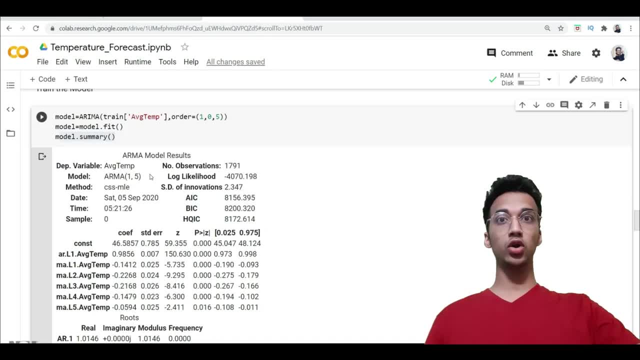 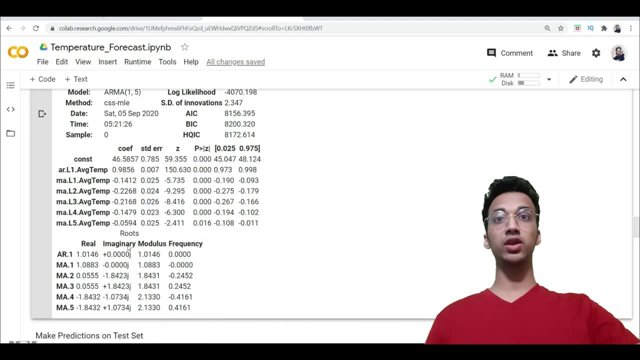 so in the summary you can see a lot of things like the aic score, the order of the model and you can see the respective coefficient for each timeline right for the auto regression of order one, the coefficient is 0.98 and for the five moving average parameters you can see the coefficient. 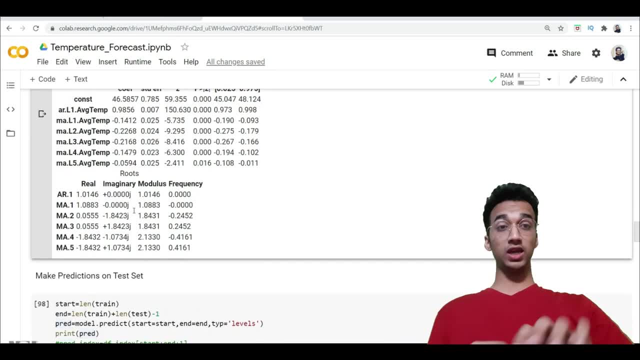 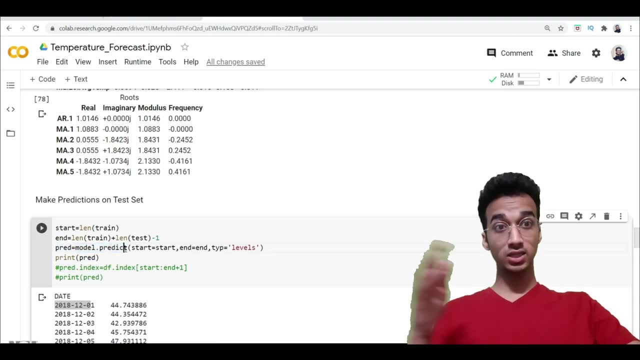 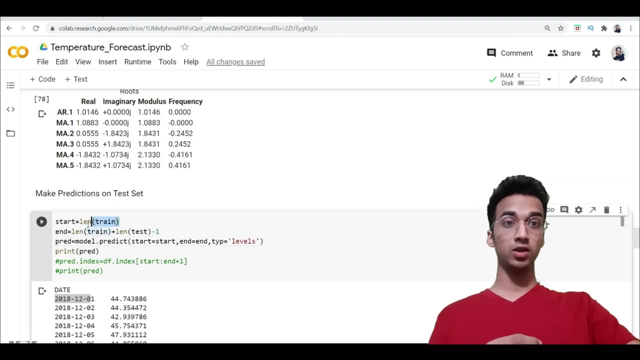 for them as well. after that, we proceed to make final predictions on the testing section, right? you do that using moldpredict and for modelpredict you need to provide the starting index and the ending index in which you want to make a final prediction for each timeline. you want to make a prediction, right, so the starting index is length of training set. 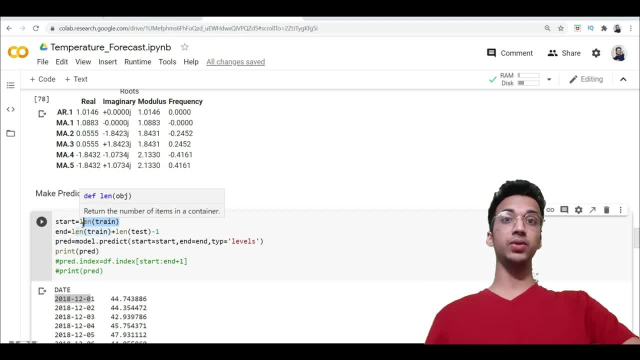 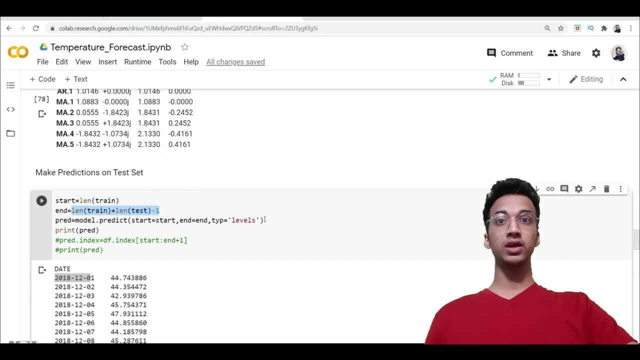 so basically, where the training set ends, from there you want to start making prediction, and it goes on till the end of the data set. all right, so you mentioned that over here in modelpredict, right and over here you print out the predictions so you can see the prediction. 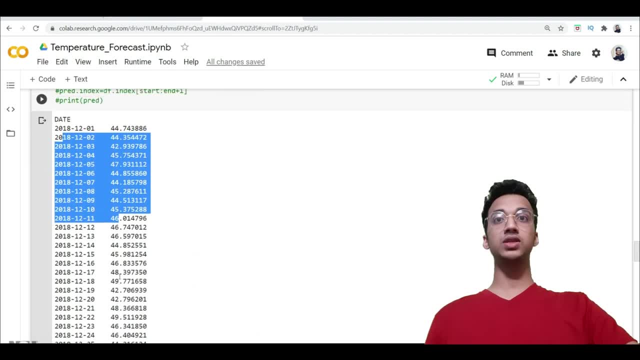 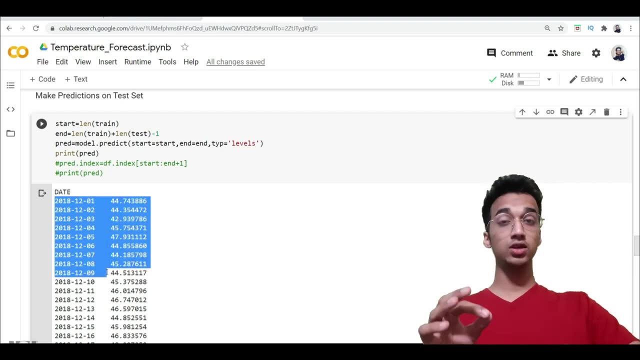 for the testing set over here. sometimes what happens is the index is not date values and instead it gives them numbers as the first prediction, second prediction, third prediction. but you always need to have dates as the index over here if you want to make a plot right, if you 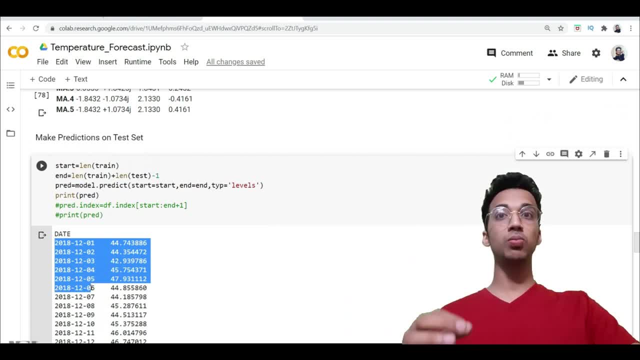 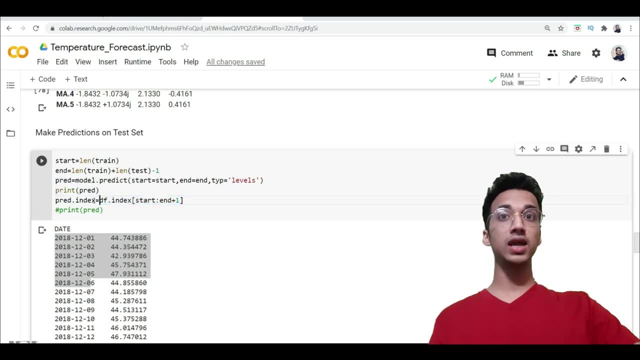 want to plot it out, you need the date values. so in some cases you might have to use this line, which is basically: uh, taking the date values from the data frame and you're assigning over here as the index of the prediction model. sometimes you might have to do this, uh, if the index is. 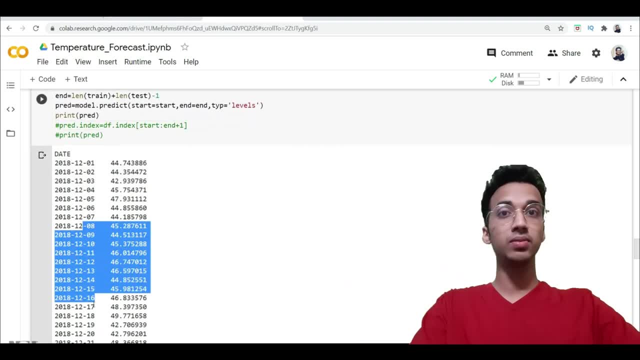 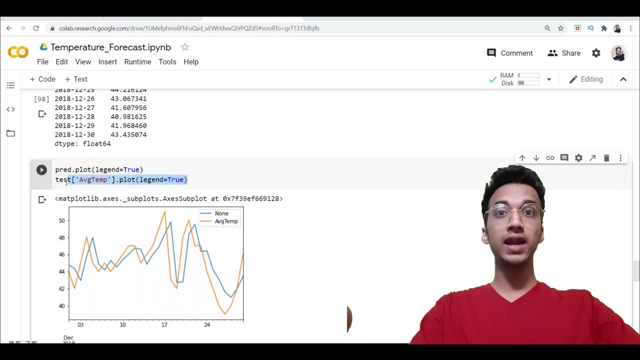 not as state over here. the index are date values, so we don't have any problem. after that we are plotting the prediction and we are plotting the test set and the prediction set and along with it to see a comparison right And you can see the model is pretty good. 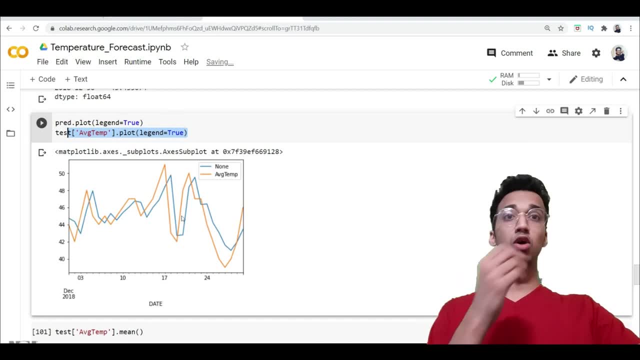 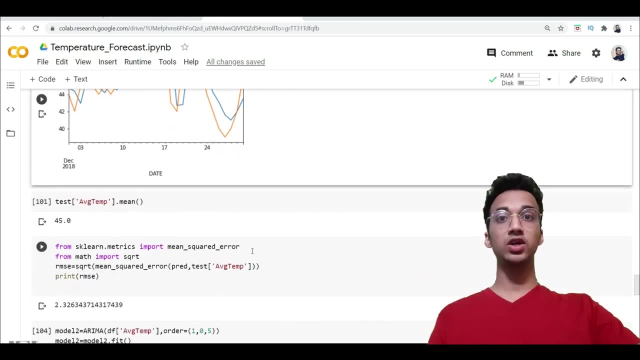 It's following the trend of the data set And if you want to see exactly how good or bad it is, you can check the root mean squared error right. So over here we import the mean squared error function from SQL or not metrics And we are calculating the mean squared. 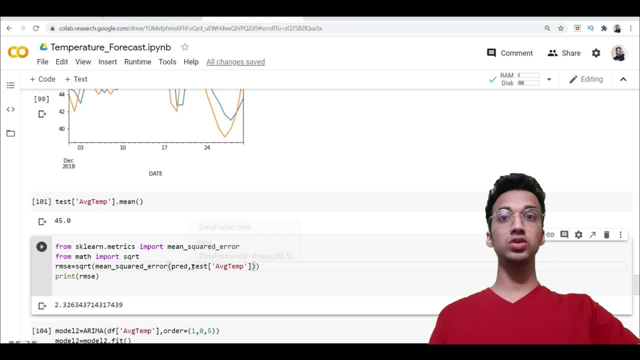 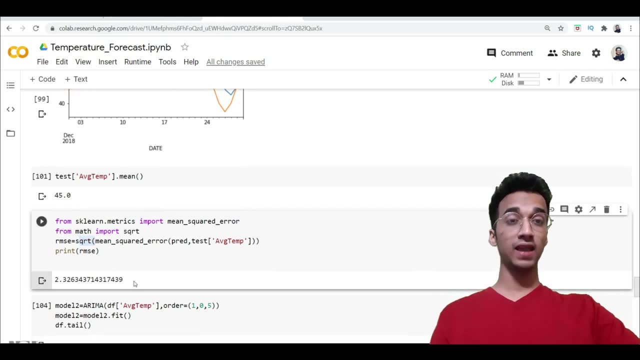 error between a prediction and the test values and taking a square root of that to get the root mean squared And the value is 2.32.. And to get a sense of how good or bad this is, you have to check out the mean of a data set right, So the mean over here is 45.. And 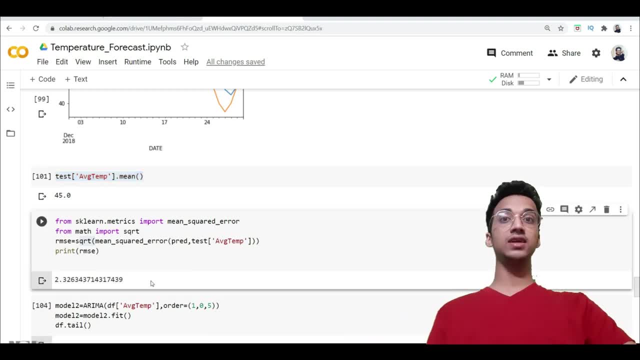 the average error is two. right, So that's acceptable. If the psi, if the root mean squared error, is very similar in range to the mean of the data set, then it becomes a bad model. Right, So that's it, we're done. But we still haven't made predictions on future values. 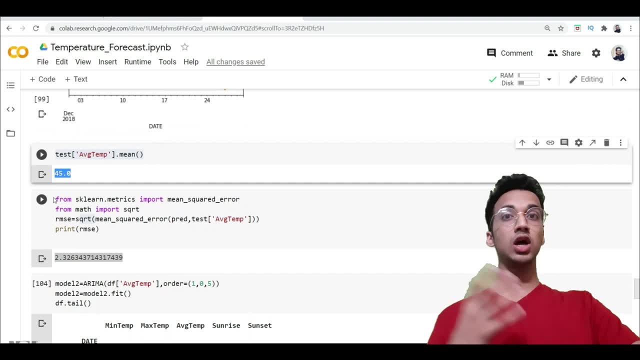 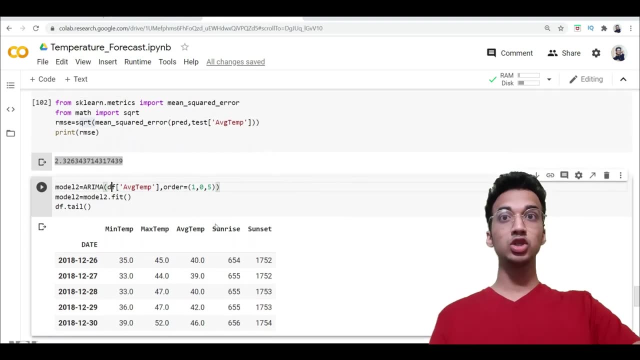 we are only making predictions on the test set so far, right. So now that we know the model is good, we retrain the model on the entire data set this time and not just the training section. So I'm printing the last five values to see at: 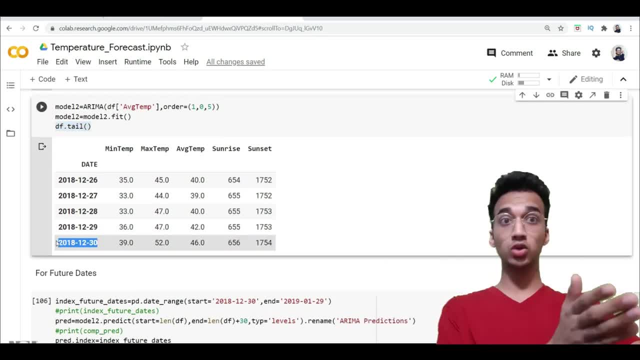 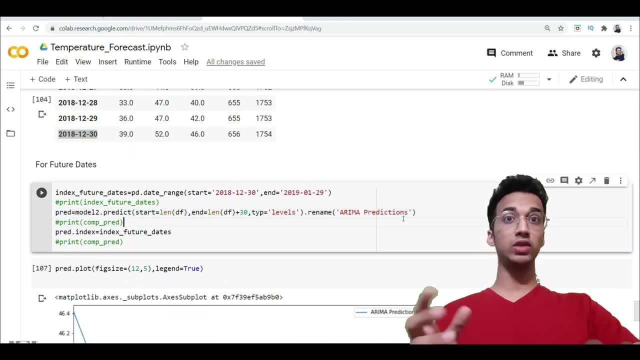 what date my data set ends And from there I'm going to make a prediction on the next 30 days. So what I'm doing over here is, again, I'm calling the model right- I'm making predictions from the end of the data set to the next 30 days. So when you actually print your predictions, 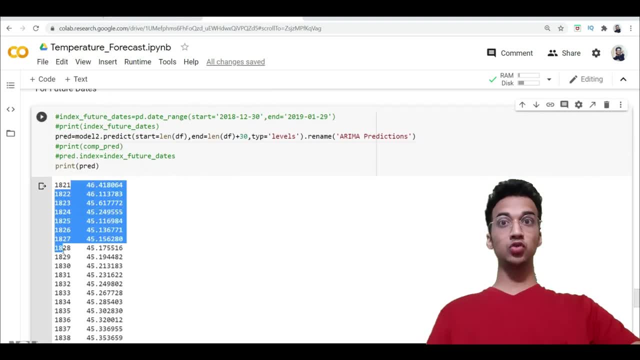 you will see that the index is not dates, right, So we simply have the number of data set. right, So we simply have the number of data set. we simply have is the 18,021st prediction. 18,022nd prediction. Now, you can't plot this. 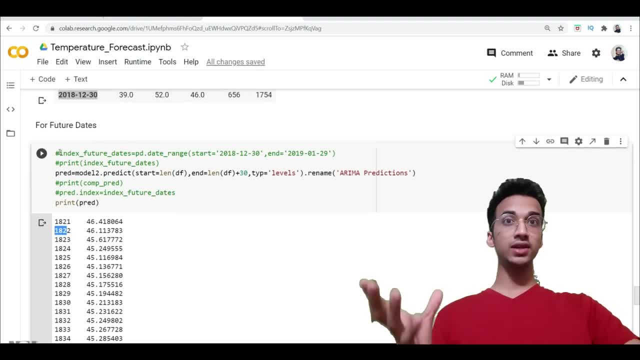 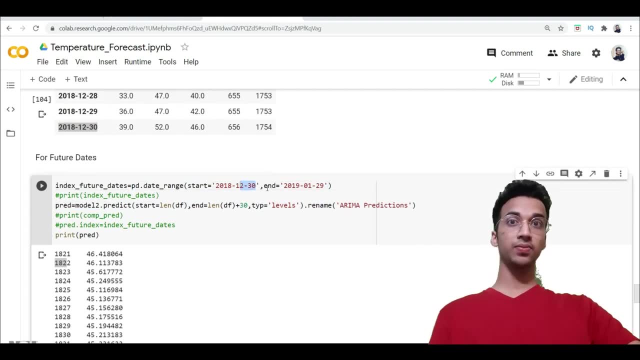 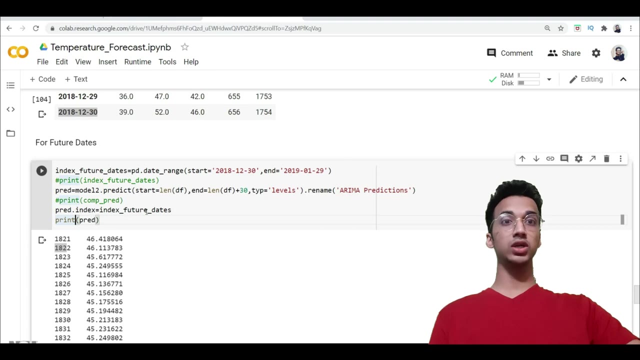 without having date values. So first, we create an index of dates, right, We create dates ranging from 2018, 30th December, to the next 30 days, And what we're doing is basically, we're basically assigning index to this prediction data frame and setting it as the future dates, right. 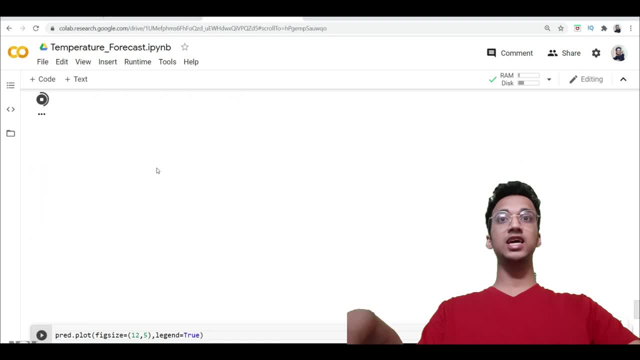 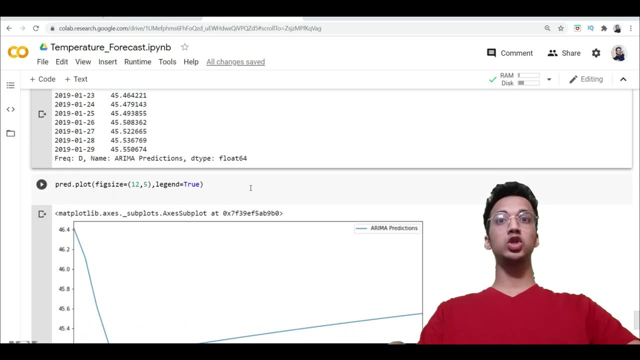 So now, if you try to print it, you'll see that the indexing has been changed to dates. Now you'll be able to plot this easily. So now, when you plot this right, you'll see this is how your future predictions look like, right? So it's basically around between 46.4. 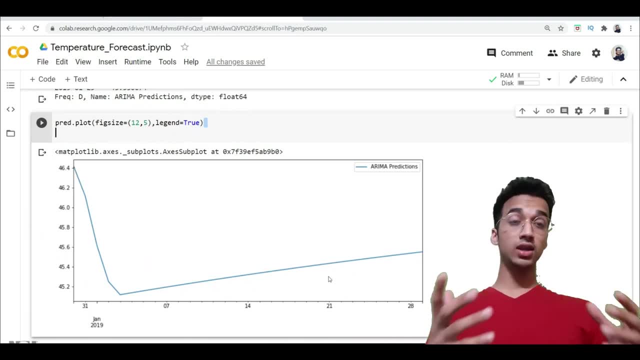 and 45.2,, I think, right. So that's how you use an ARIMA model And that was all for this video. In the future videos I'm going to talk about different models and how you can use that for more complex time predictions. So if you did like this video, do like it. and subscribe to this channel. And yeah, thank you for watching.